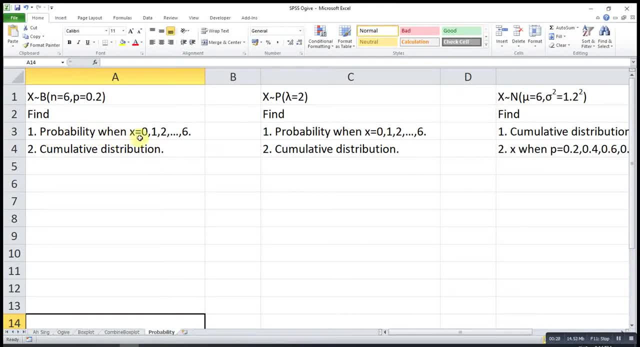 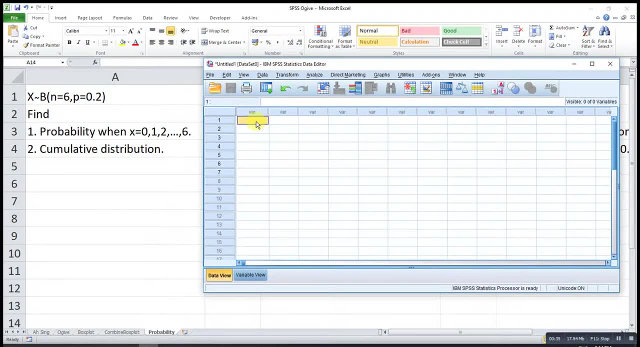 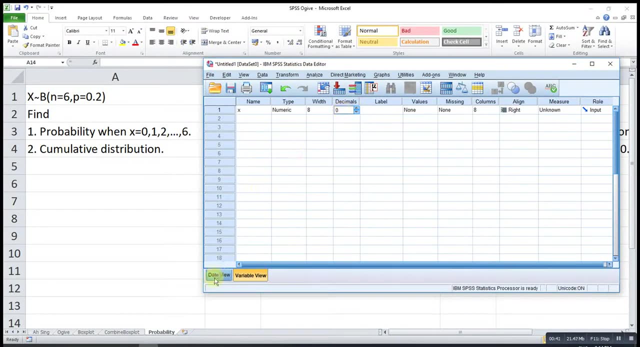 If let's say, we are asked to find probability when x equal to 0,, 1,, 2,, 3 and so on. So what can we do here? First, input the value of x that needed. So under the variable view here we can give a name of x with 0 decimal. 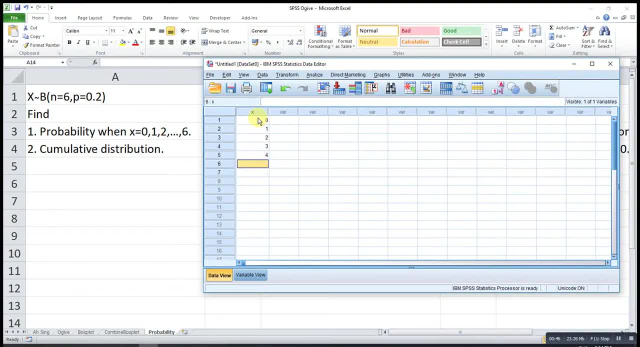 So we need 0,, 1,, 2,, 3,, 4,, 5,, 6.. Then after that go to transform compute variable. Then under target variable here we can give any name of the output that we like. 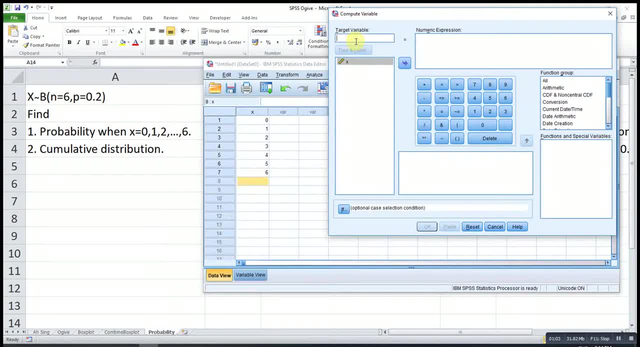 So we can type probability or probability distribution or just simply pdf short form probability density function. We have to bear in mind that we cannot put any space here, Otherwise we will result an error. So look for probability density function binomial. 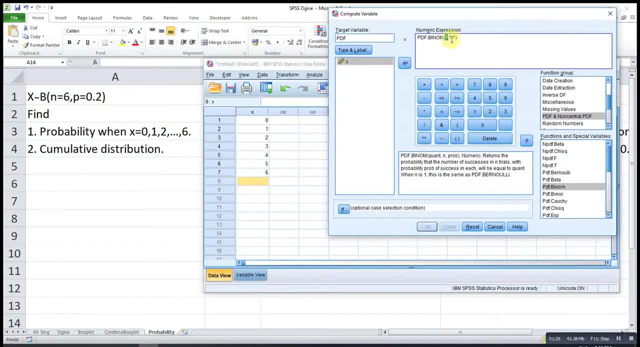 Then we select. Okay, we have 3 question marks here. The first one is the 1.. So it's the variable. Then we input: the second question mark is the n, So number of trials that we have 6.. 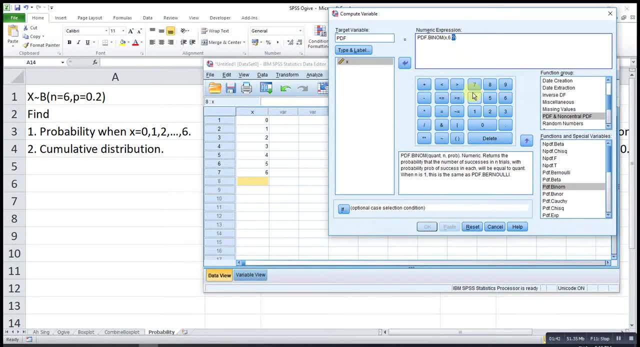 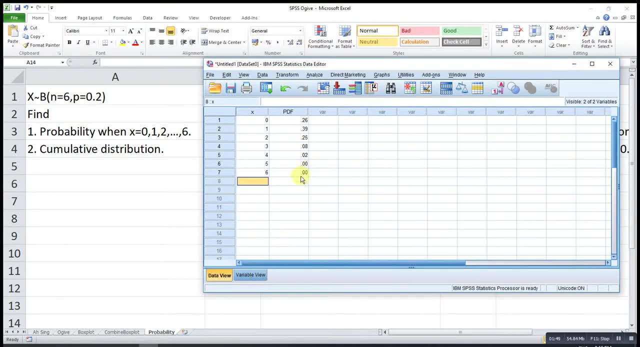 And the last one is: the probability means that the success rate 0.2.. Then okay, So the probability already computed. So let's say we want to increase the decimals, We can go to variable view and increase accordingly. So let's say we are asked to find the cumulative distribution. 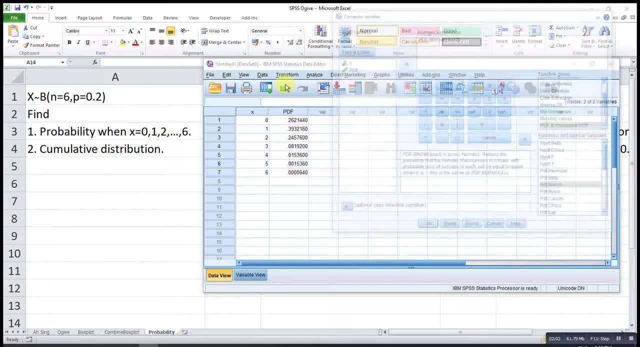 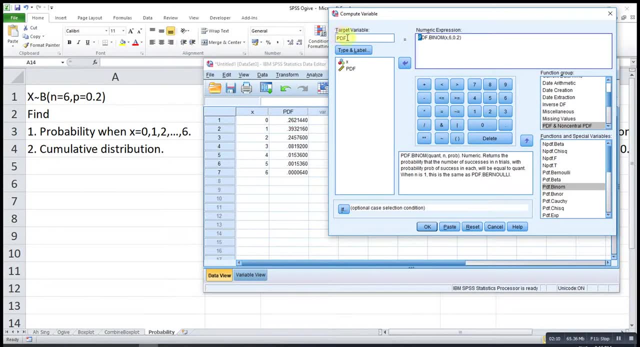 Also go to transform compute variable. Okay, we can simply change p to c. Let's say, we worry any error arises, Then we just delete. Then we look for cdf binomial, Then we select: Okay, as we can see change from p to c already. 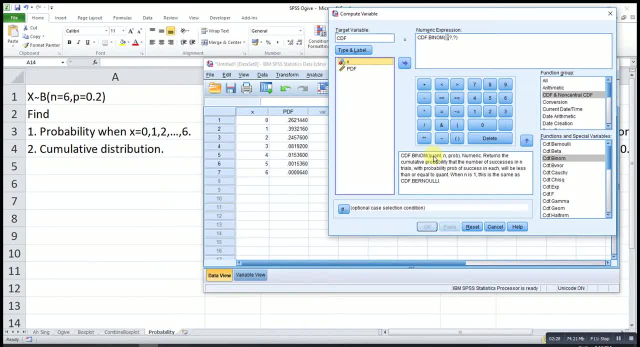 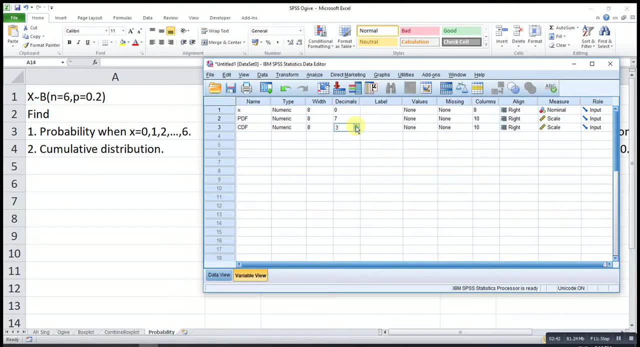 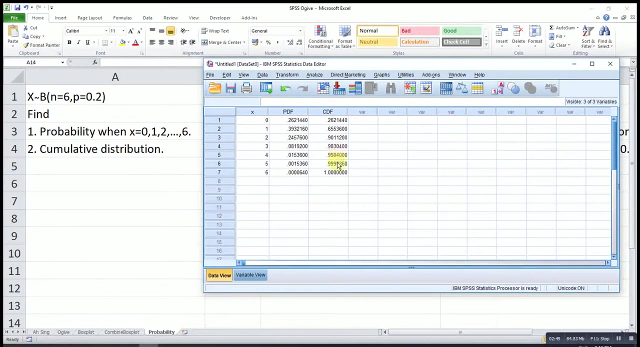 Okay, Also, the first question mark is the 1.. Then second number of trials is 6. And then the last one is 0.2. Okay, Also, we can increase the decimal places. We have to bear in mind that the numbers here or the probability here, 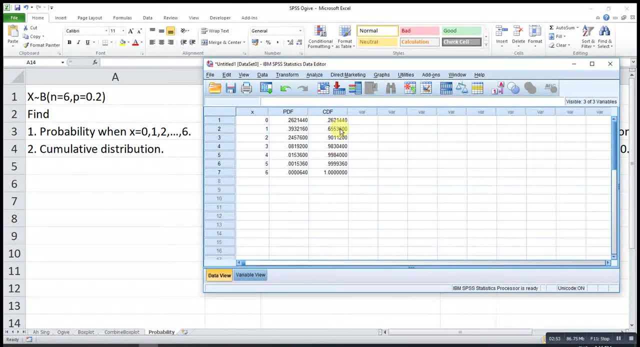 Actually sum is the sum up to the number. that indicated Here Means that they are respective number. So let's say the cdf for this row is the probability that sum up to 0.. And for this one is sum up to 1.. 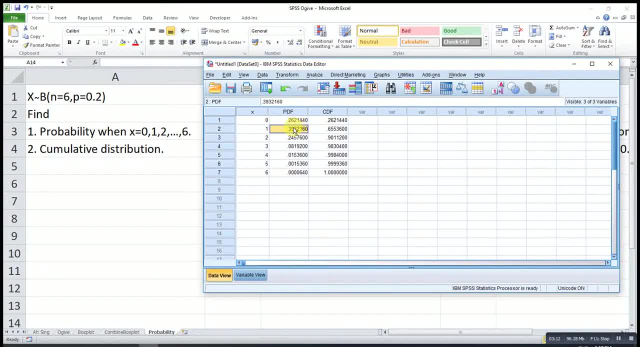 So means that we take this number plus this number, We will have this number, And we take the sum of these three And we will obtain this. Now let's do the same thing for Poisson distribution. So for Poisson distribution. 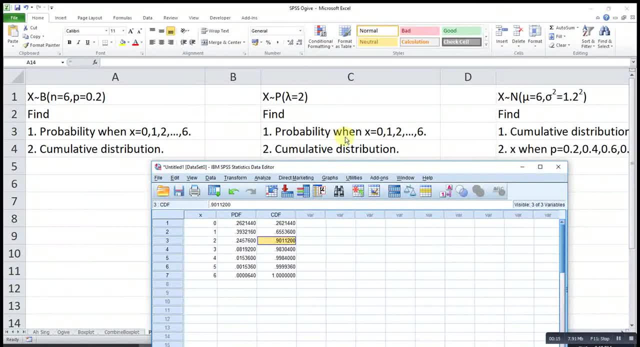 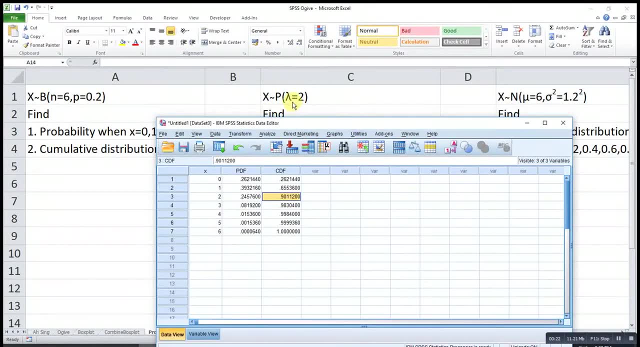 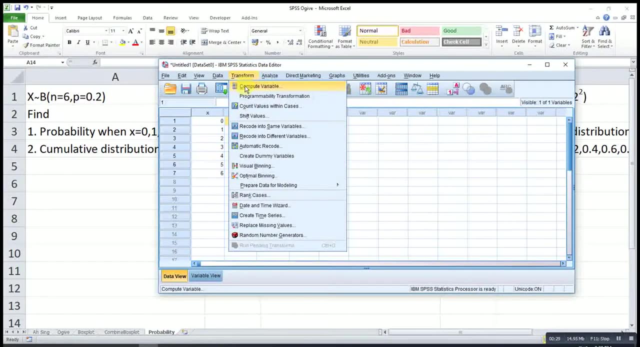 We are asked to find probability and cumulative distribution Then for x, 0 to 6.. So with means equal to 2.. Lambda equal to 2.. Okay, Delete these two. So transform compute variable. Okay, Change to pdf. 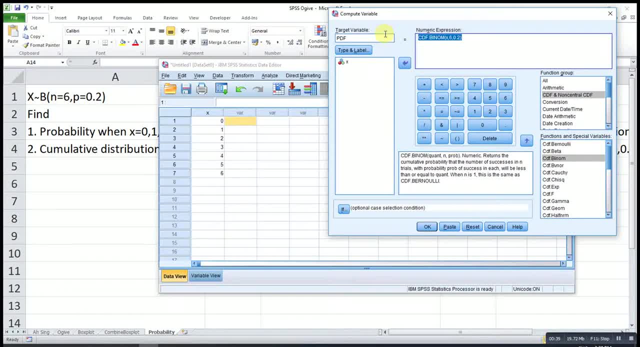 This one is now for Poisson distribution. So we look for pdf Poisson Poisson, Then we select, So we have 1 and mean, So quantity and mean 2.. Mean is the lambda, So okay. 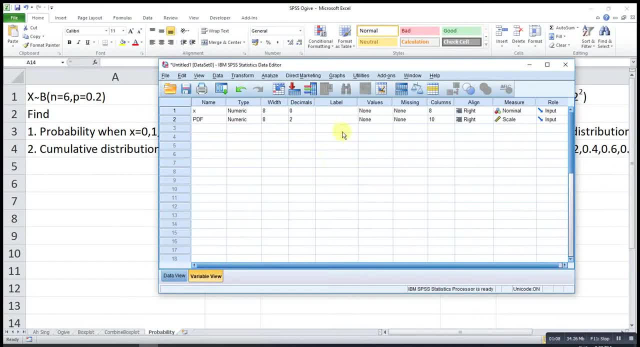 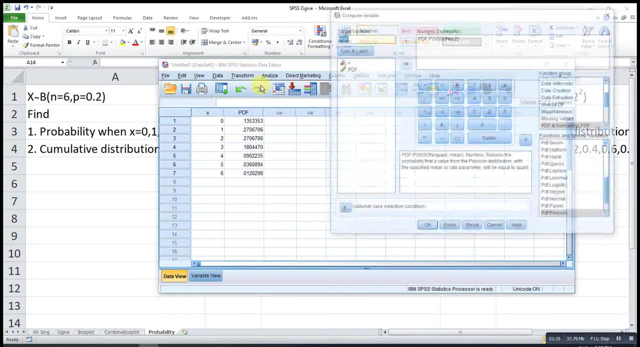 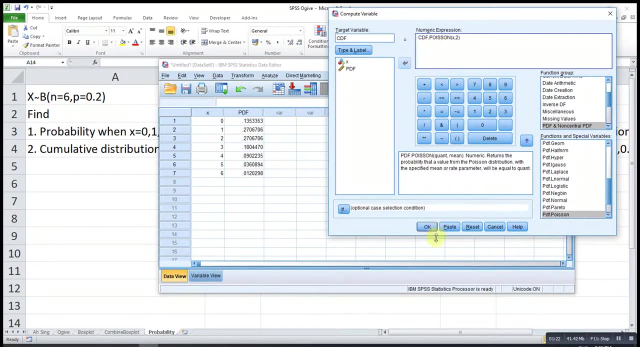 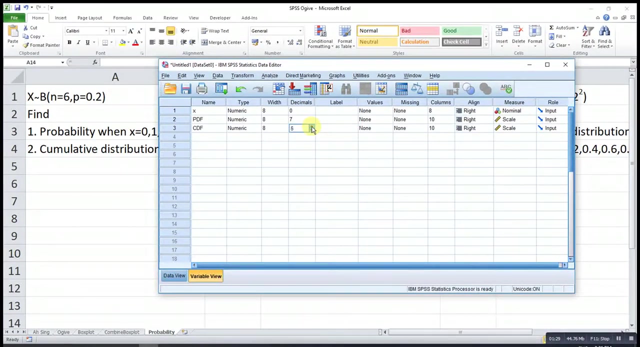 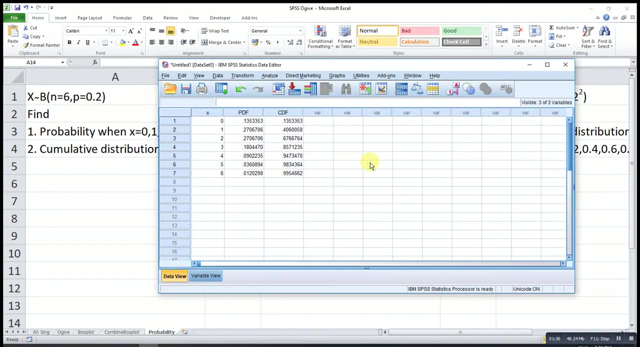 Then we done Okay. Can increase the decimal places? Okay, Now do for cumulative Change: p to c, P to c, Then okay, Then we done Okay. Now let's try for normal distribution. For the normal distribution. 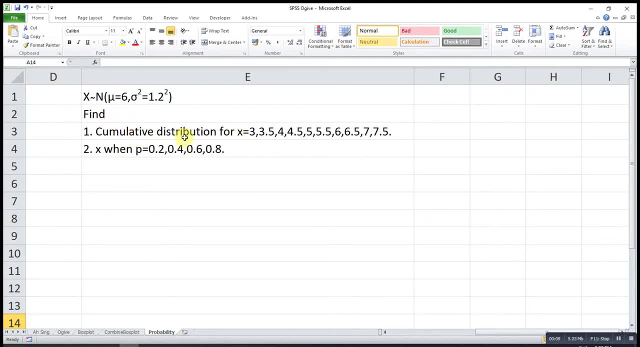 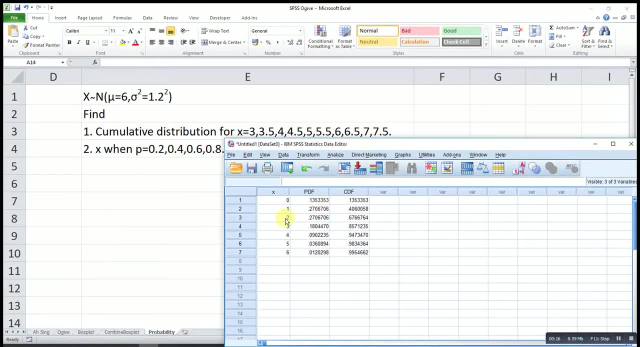 So we are asked to find the cumulative distribution for the value as all these. Okay, So we just type accordingly. So delete these two, So we 1, 3. Then 3.5. 4.. 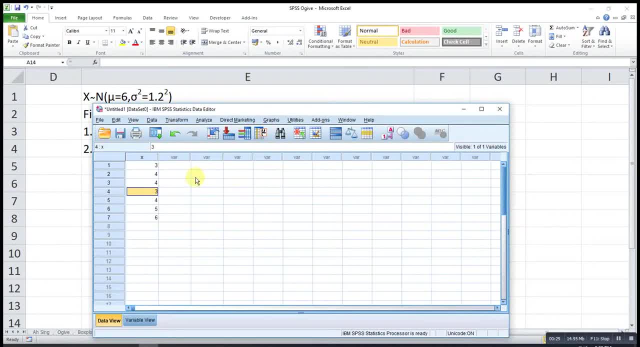 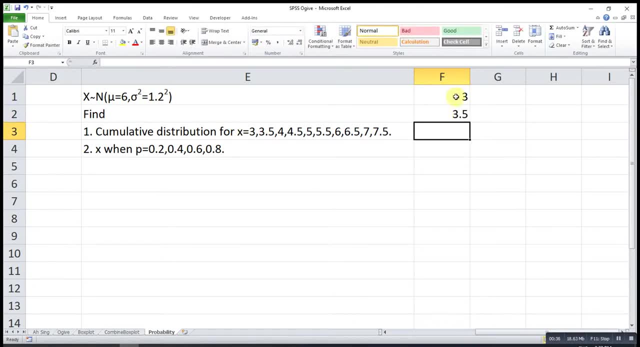 4.5 and so on. Let's say we lazy to type one by one, So we can make use of excel. So what we need is 3. Then, followed by 3.5, and increase 0.5 for each. 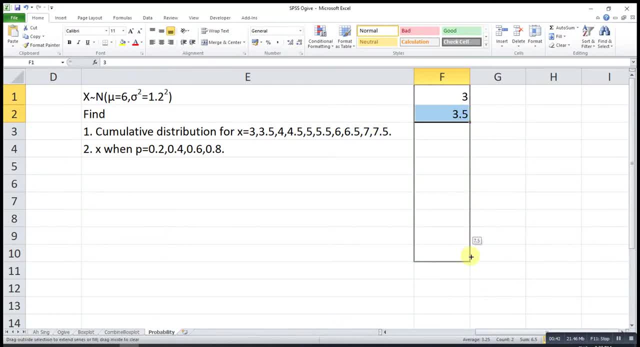 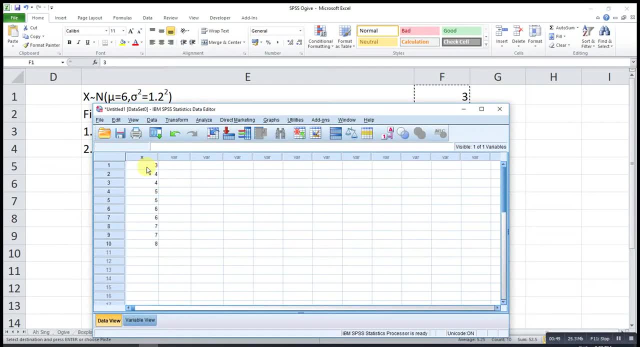 So we just drag until we have 7.5.. After that we just copy and paste to SPS. So remember to change to decimal one. decimal, Okay. So we first find the cumulative distribution, So transform. 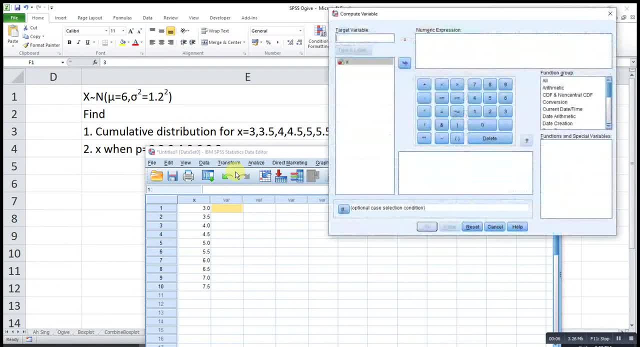 So transform Compute variable. Look for CTF, Then look for normal distribution, Normal Select. Okay, For the first one is the guan. Okay, Before that, remember to write the name CTF. Okay, The first one, guan. 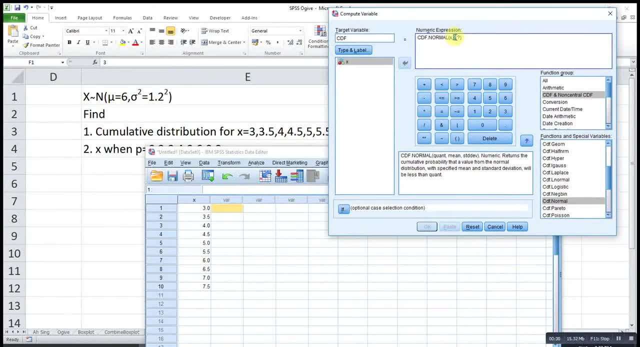 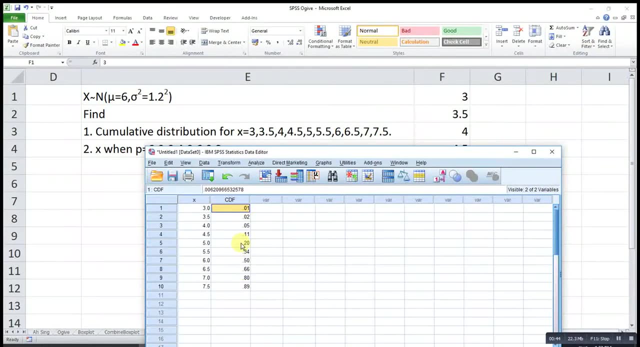 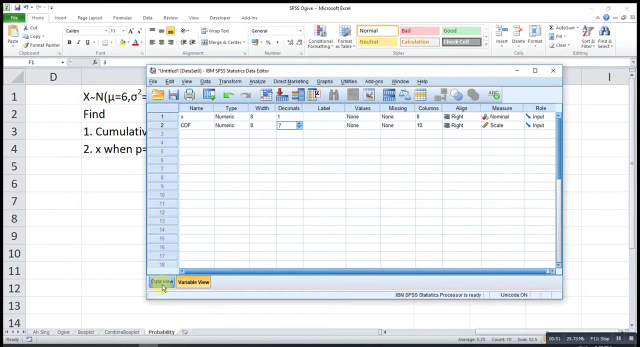 Okay. Second is the min Means that the mu 6.. The last one is the standard deviation. Standard deviation 1.2. 1.2.. Then, okay, So the probability already computed. Okay, We can change the number of decimal places according to our preference. 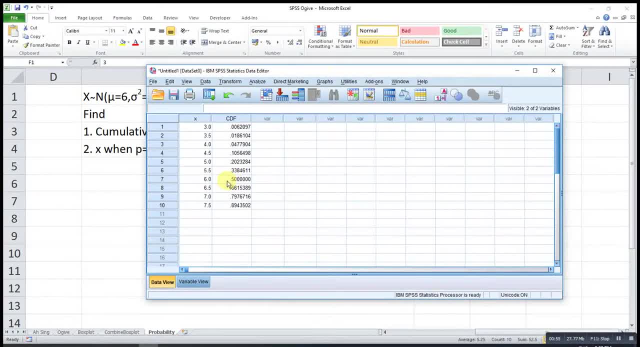 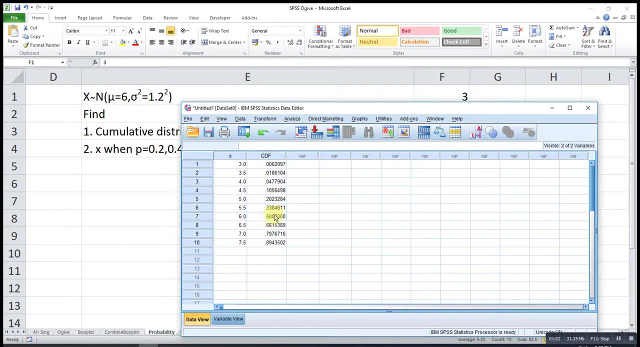 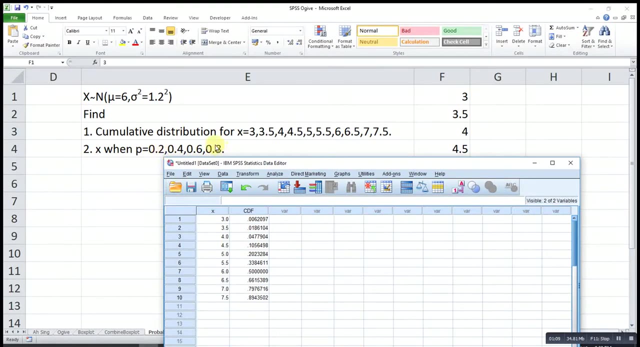 Okay, We can see here: 6 is 0.5.. Okay, Because the min is 6.. So the grand x equal to 6.. We should have 0.5.. Okay, So the next one is to find x when p. okay, are given all these. 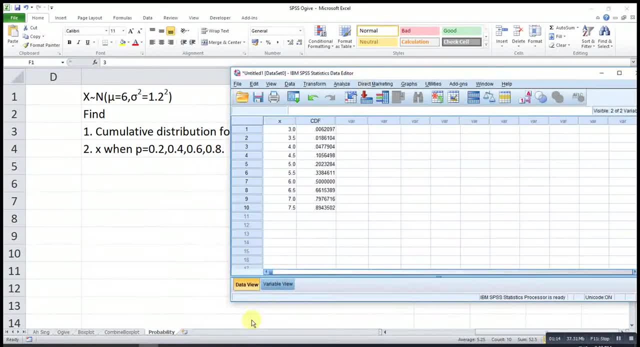 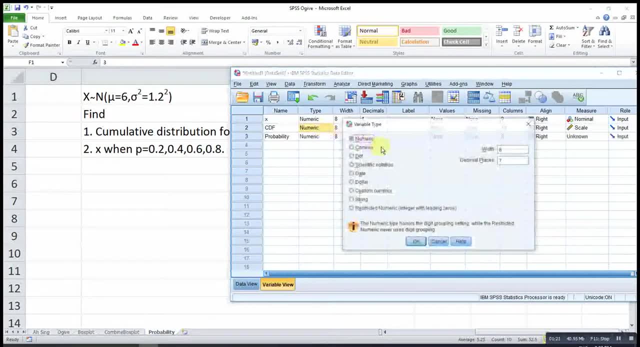 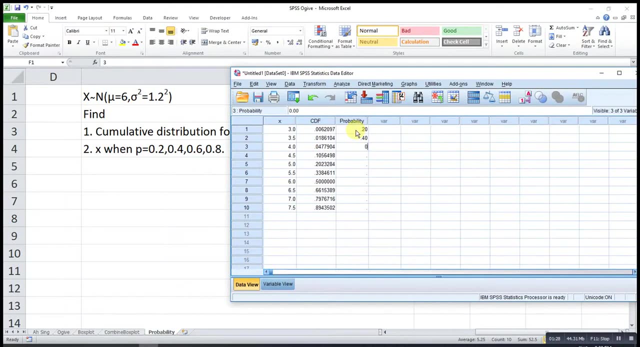 So what we need here is we are given the probability, Probability and ask for x, So probability, leave it to decimal places, So 0.2, 0.4, 0.6, 0.8.. 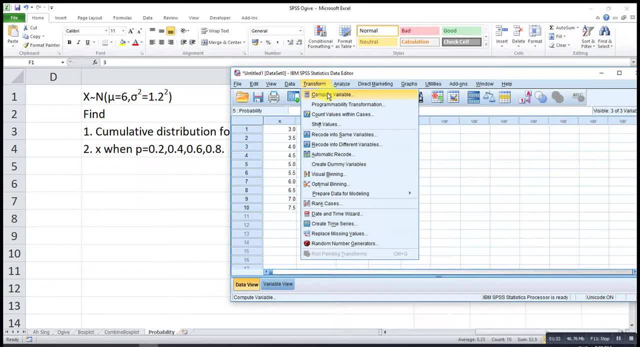 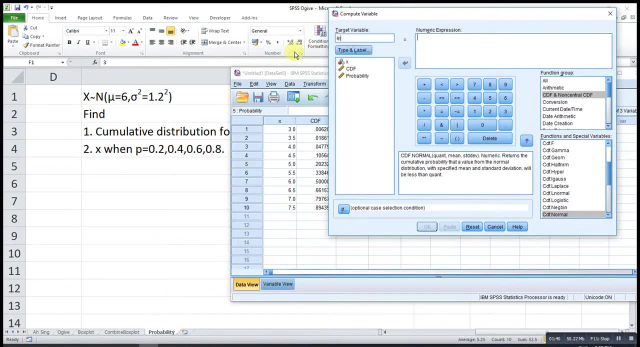 Then transform Compute by apple. Now we should look for inverse, Since we are asked to find the inverse function. Inverse, So inverse, df, Normal Select. So the first one, the probability Stick, that here. 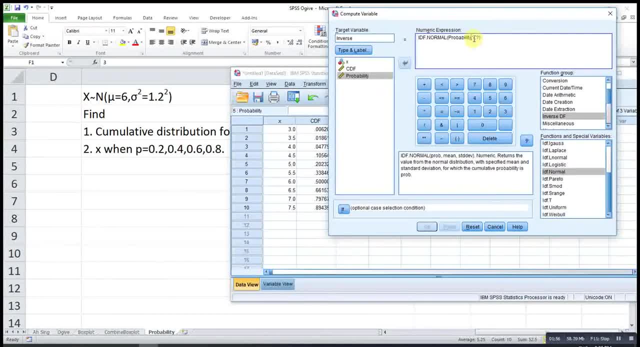 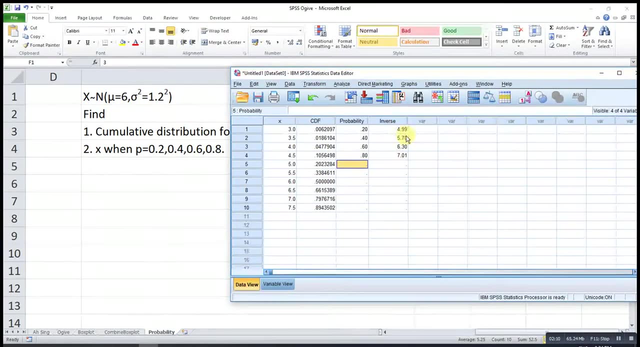 Probability, Then followed by min: Min is 6. And standard deviation And standard deviation 1.2.. Okay, Then the value of x, already obtained here. Okay, That's all for today. Thanks for watching. Hope you like this.